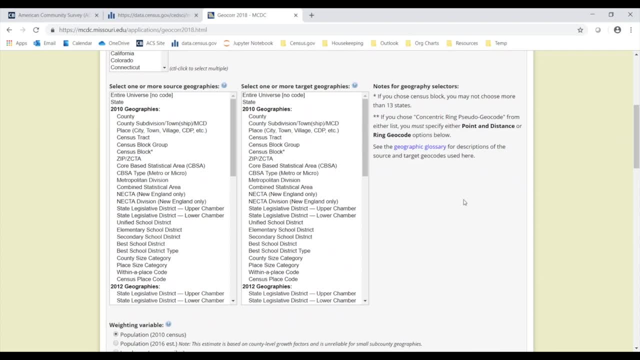 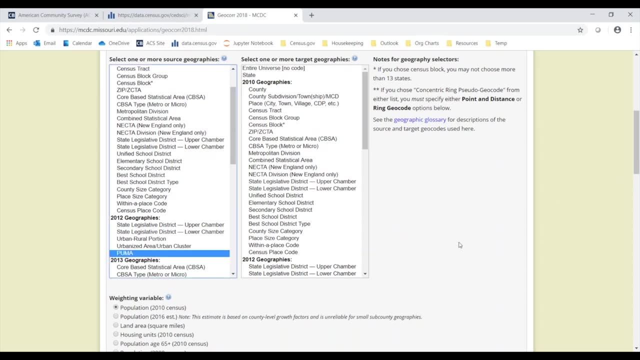 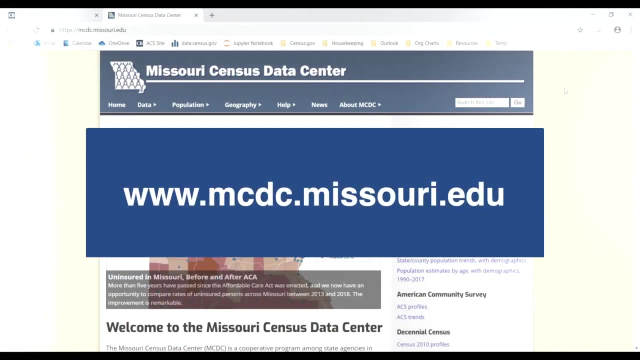 type of geography to another. We will use this tool to make sense of a particularly unusual census geography: the Public Use Microdata Area, or puma. Let's see how it works. We can navigate to the software through the Missouri Census Data Center website at mcdcmissouriedu. 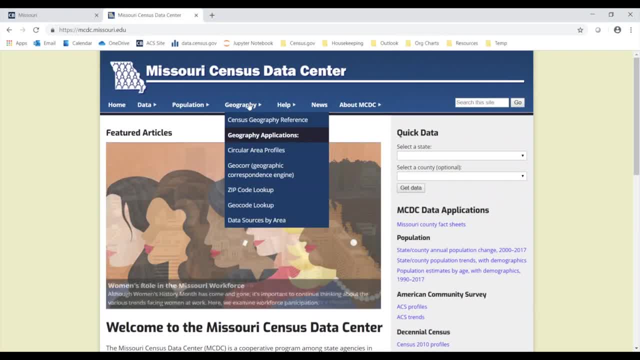 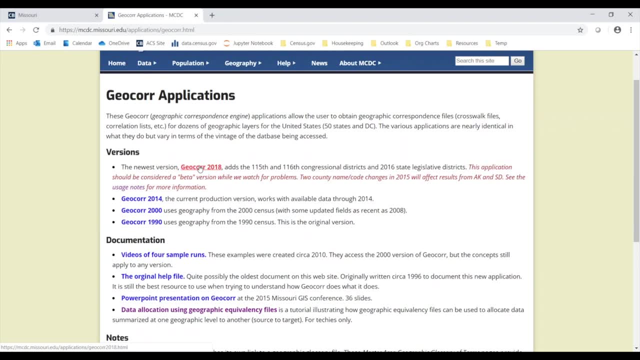 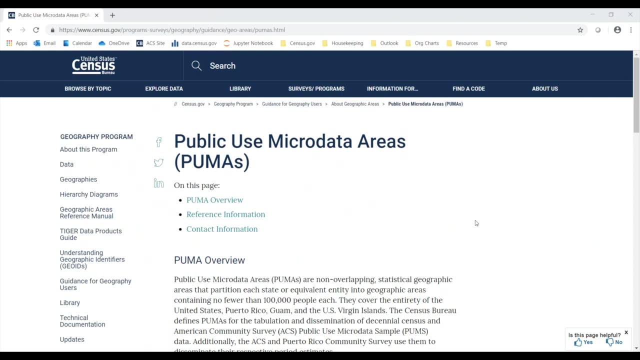 From the landing page, hover over Geography and click on the GeoCore option. On the next page, click on the GeoCore 2018 link under the version. Our users often work with a geography called Public Use Microdata Areas, or pumas, so that 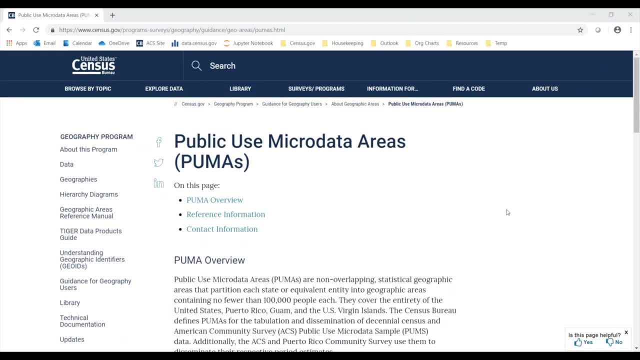 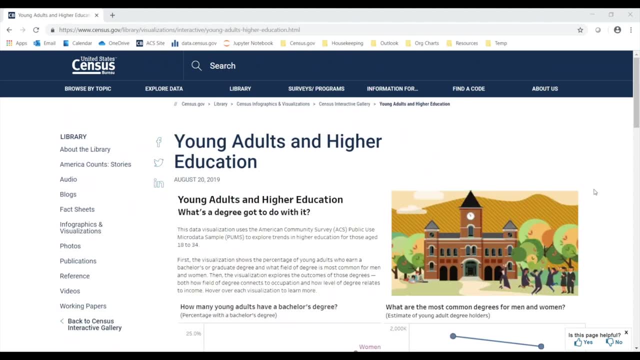 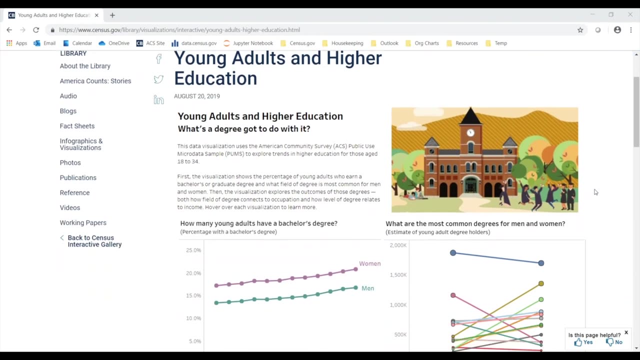 is what we are going to be working with today. Certain census datasets, such as the American Community Survey's Public Use Microdata Sample, use a type of data called microdata. Microdata allows users to create custom tables, such as the ones used to make this data visualization on censusgov, on young adults and higher education. 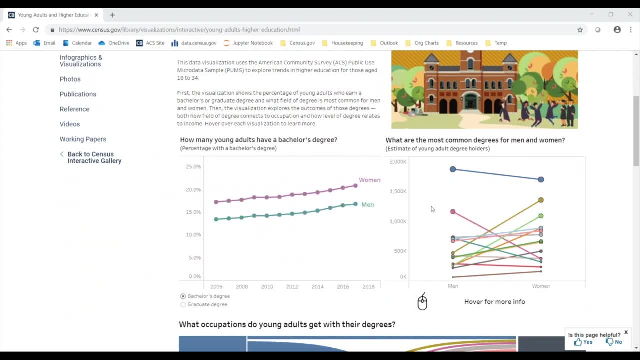 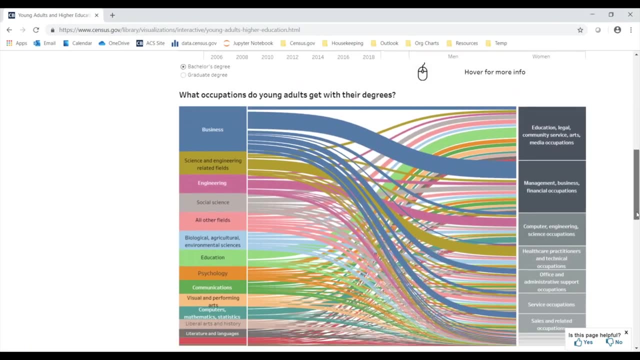 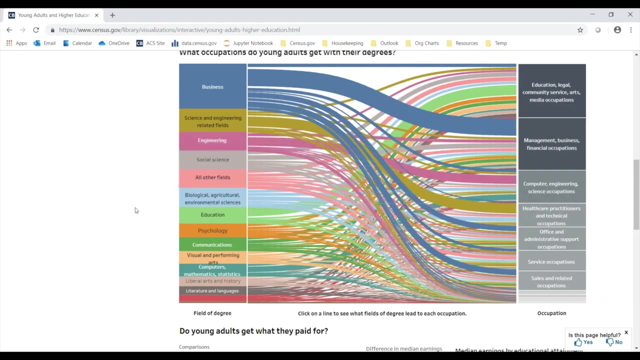 This allows users to learn things about their community that aren't always readily available in a premade table, such as the age and race breakdown of a particular occupation or the characteristics of children below a certain poverty level. GeoCore is useful for working with datasets like these, because people often have to find 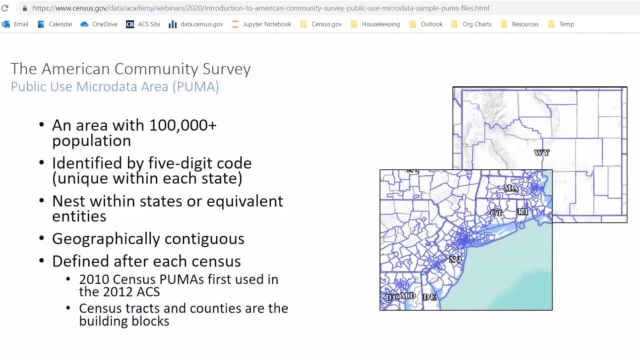 information using pumas. but there are good reasons why pumas are used with microdata. Pumas are areas with a population of at least 100,000 and more. We can take the data coming from, let's just say, the applicants for a census or a census. It can include all of the data. 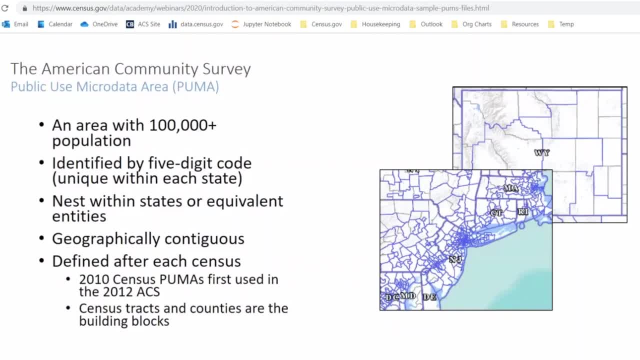 that we have gathered throughout our survey. We can also find different information: that which is small enough to give users useful local information, but large enough to protect the privacy of people who respond to our surveys. As with anything related to geography, seeing pumas on a map may help you understand them better. 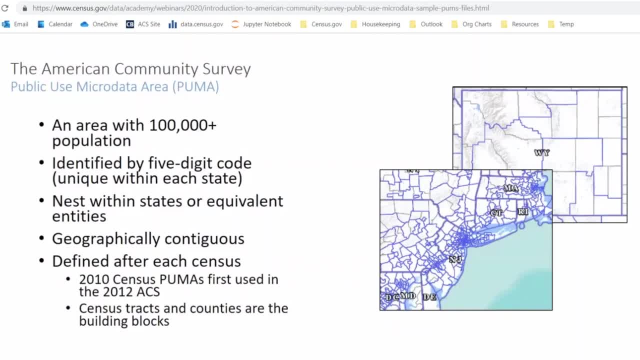 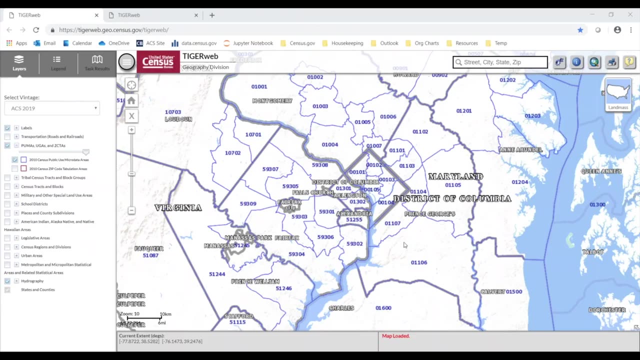 These two maps are shown at the same scale. You can see that most of the pumas in Wyoming are larger than the pumas in New Jersey. This emphasizes that pumas are truly built based on population and not on physical size, Since pumas contain approximately 100,000 people, regardless of where they're located. 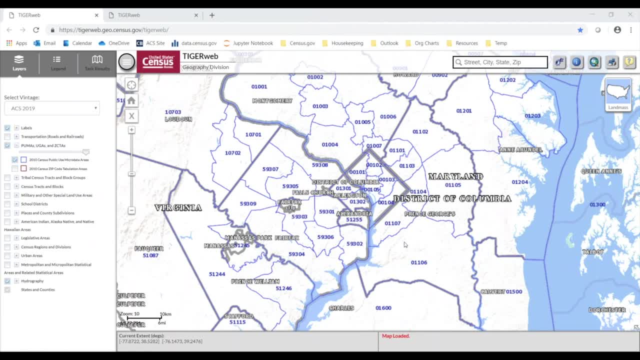 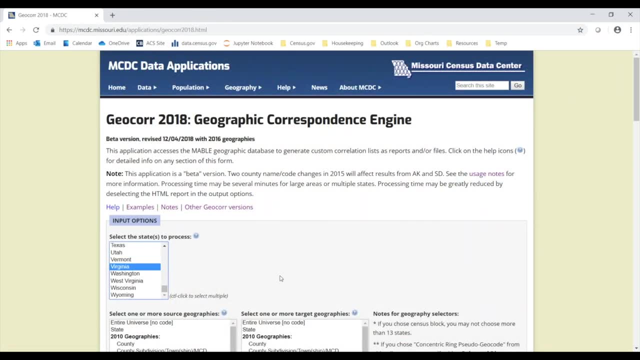 you can probably imagine that more urban counties are made up of many pumas, whereas more rural counties could have several counties in one puma. Now that we've compared pumas to a more familiar geography, we can see how this works in GeoCorps 2018.. 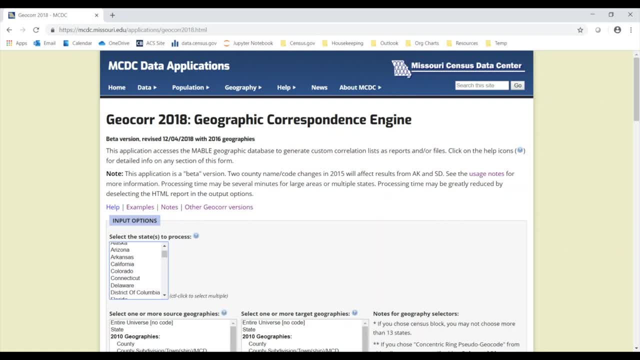 Once on the GeoCorps 2018 page, we are going to select our state. For this example, I will select the Census Bureau's headquarters home in Maryland. If I hold down the control key, I can select more than one state, so I will select a neighboring state- Virginia. 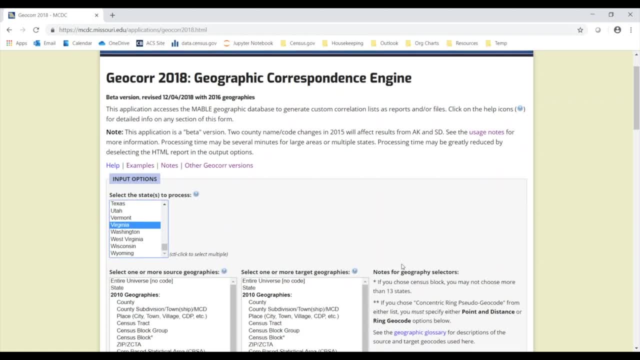 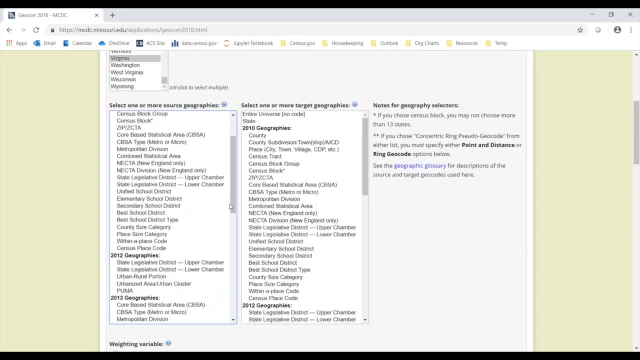 Down in the geography selections you can see there are a lot of geographies to choose from. The source geography is the state of Virginia. It's the geography you want the software to start with, And the target geography is the geography that you want to compare to the source. 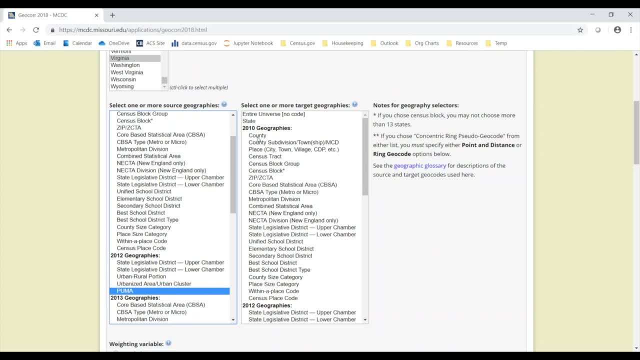 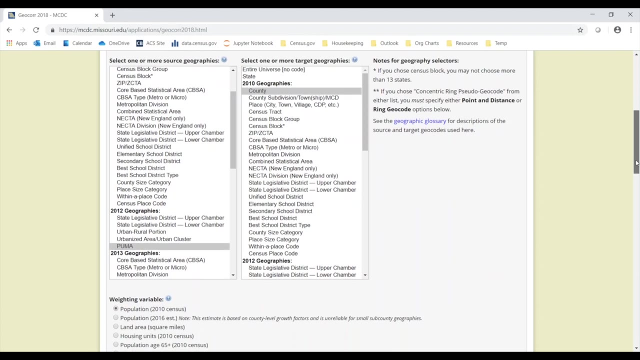 We're working with pumas, but we want to know how that would translate to counties. You can find puma under 2012 geographies and county under 2010 geographies. That just means that these were the years the boundaries were established, based on information from the 2010 Census. 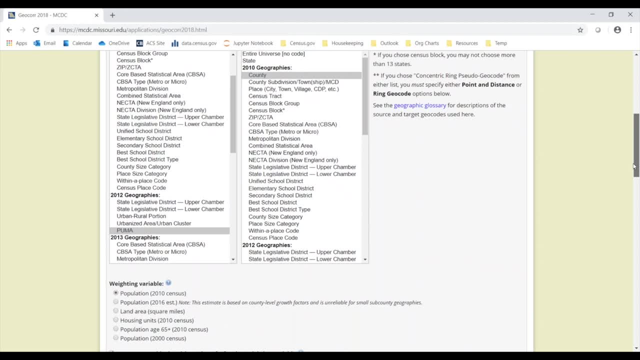 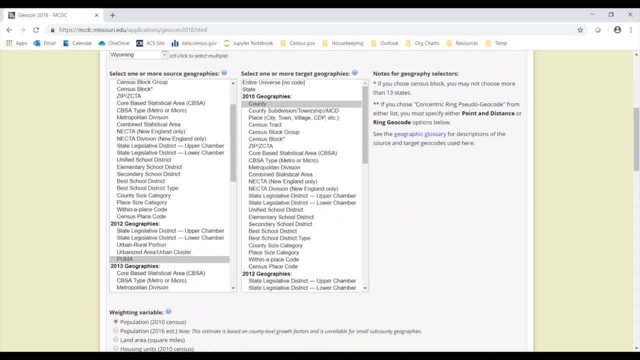 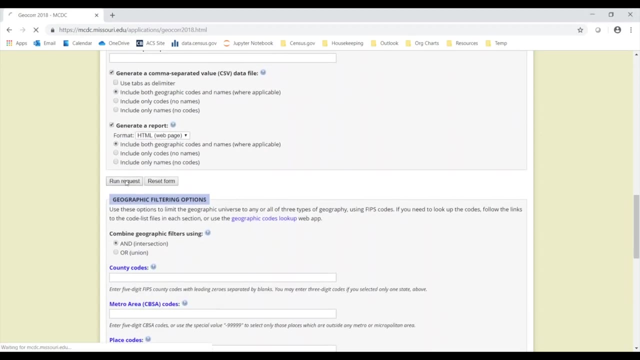 When working with pumas, I find it useful to always start with pumas as the source geography- In this case county- will be the target geography. We'll keep it simple today and leave everything else as is before we click on Run Request. 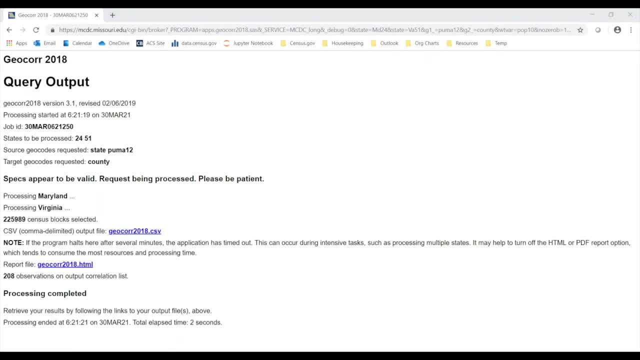 You can now view this report as a CSV file using programs like Excel, or you can view it in your browser. Today, we will view it in Excel. You can just click on this first link and it will download. Go ahead and open it in Excel. 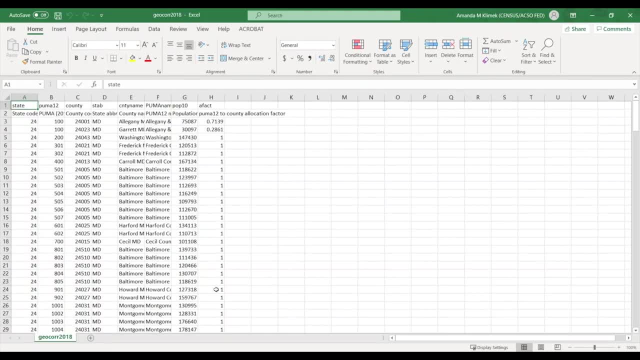 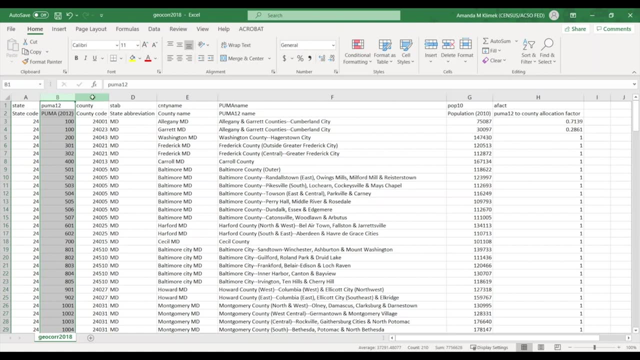 And here is our comparison. Here we have the state code in column A, the puma code in column B, the county code in column C, the state abbreviation in column D, the county name in column E and the puma name in column F. 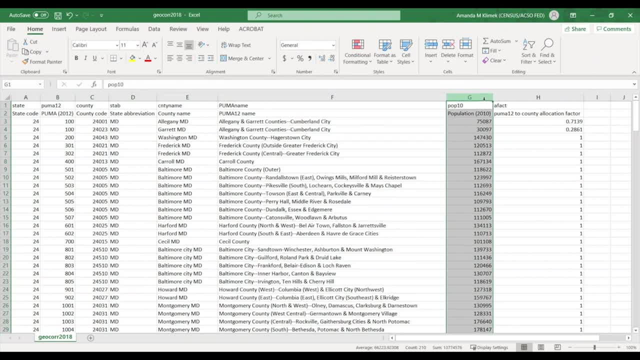 Column G gives us the 2010 county population, which is what our file is using to do the geography conversion. In column H, the variable AFACT is called the allocation factor. It shows us how much of the puma is located within the county. 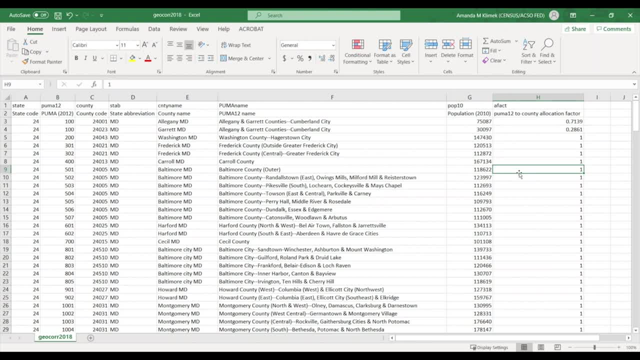 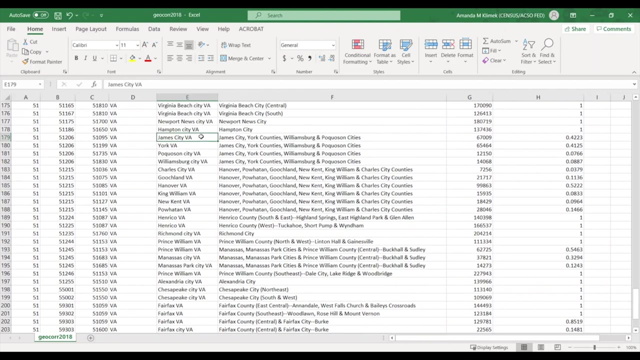 A cell value of 1 means that 100% of the puma is located within that county. We see a lot of 1s in Baltimore County, meaning that those pumas fit neatly within the county. But if we scroll down we see that James City County, a smaller county where the historic Jamestown settlement was founded- 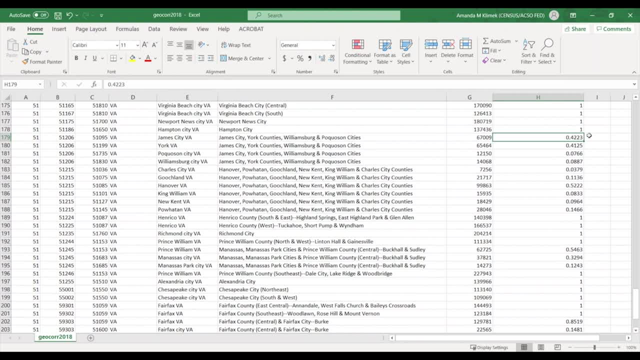 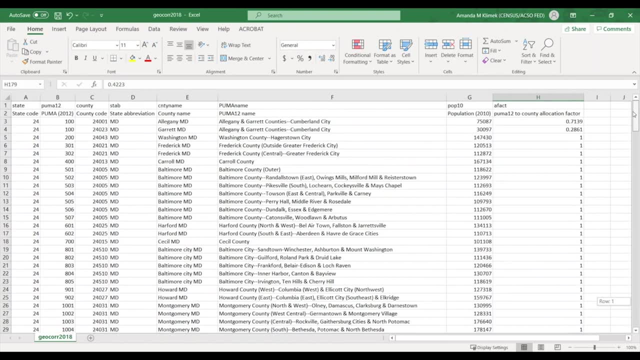 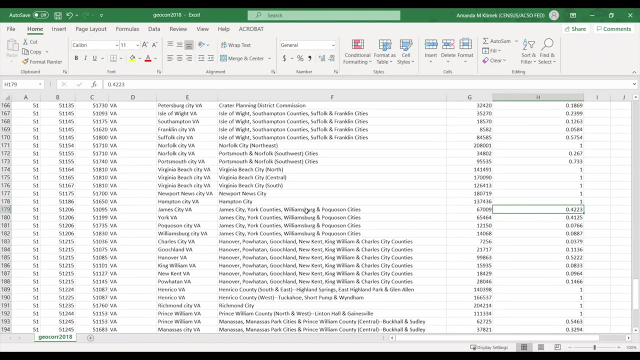 only makes up 42% of the surrounding puma. This means that we could combine the pumas in Baltimore County to get approximate employment information for that entire county. But if we want to find employment information for those living by Jamestown we will have to include the surrounding counties as well. 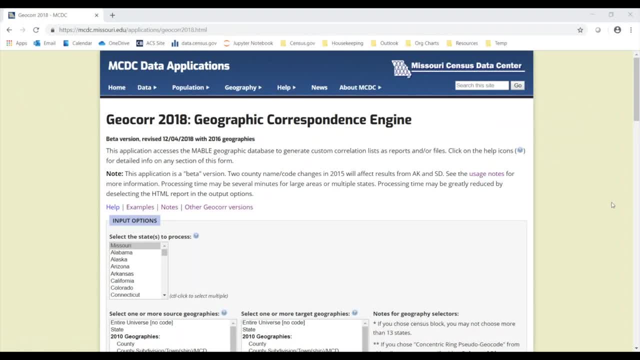 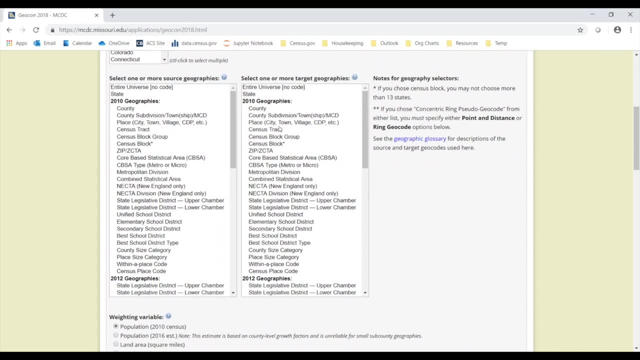 I hope that this data gem was useful to help explain the key features in GeoCorps 18 and the basics of pumas. As you saw in those extensive geography lists, you can use this with other geographies too, For instance, if a county started collecting a new tax and you wanted to know how much of a state-legislated district was affected by the new tax.